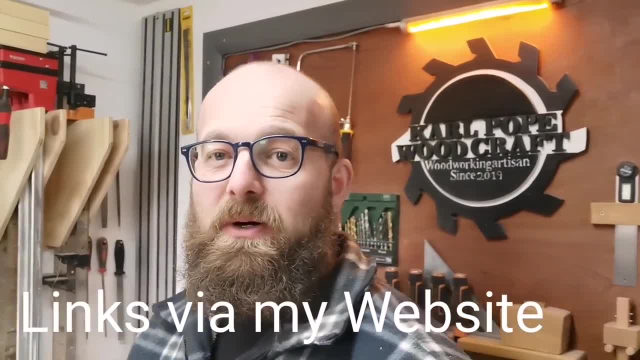 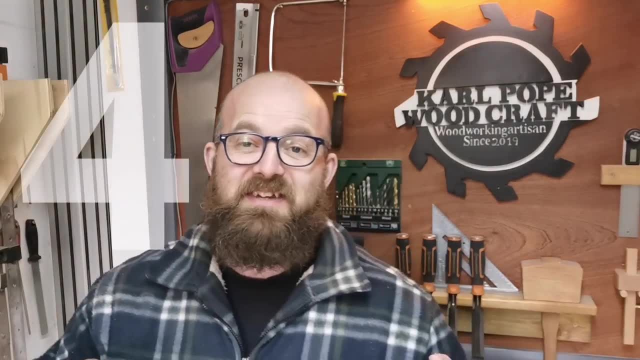 that's one of my best finishes for these: Quick, easy, simple and they're a great seller. So that's my number 5 most popular item at the moment. Coming in at number 4 then is an even easier project: shelving. Now I've got one up here that I use just to dump loads of accessories on in my work. 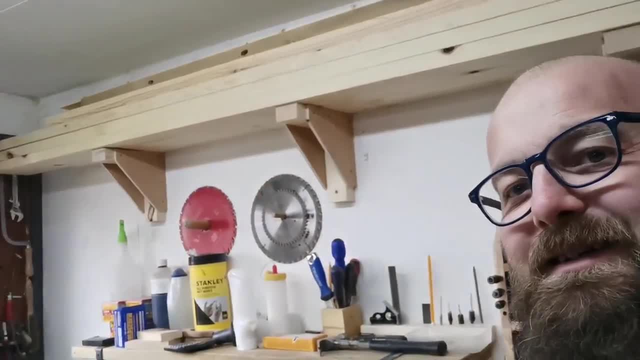 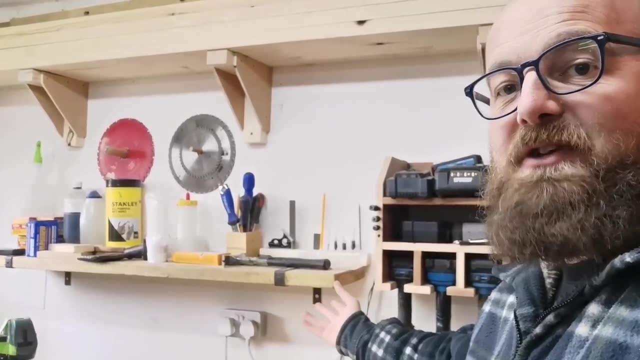 shop. I'll quickly show you that. So there's one that I've got in my work shop. you can see, it's just a piece of scaffolding board with some industrial style brackets on again. you can find loads of supplies of these on the internet, but all you have to do is cut them down to the dimensions. 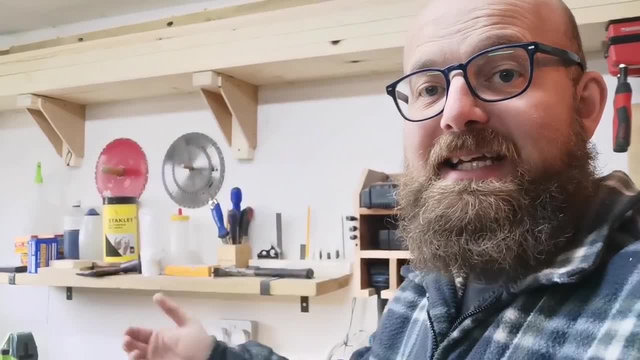 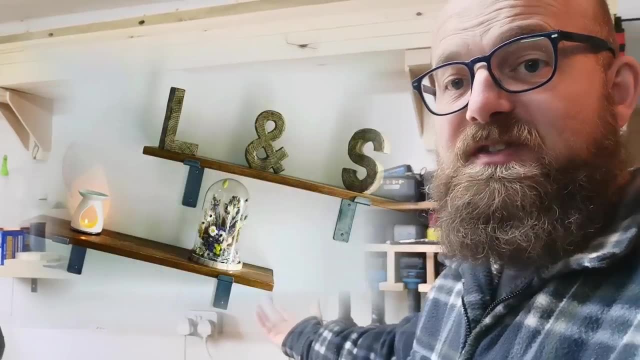 the client wants, or you can just sell them as set dimensions, say, on a website like eBay or Etsy. all you have to do is rub them down to 80 grit, put some wax on and get some industrial brackets. there's loads of supplies out there online. 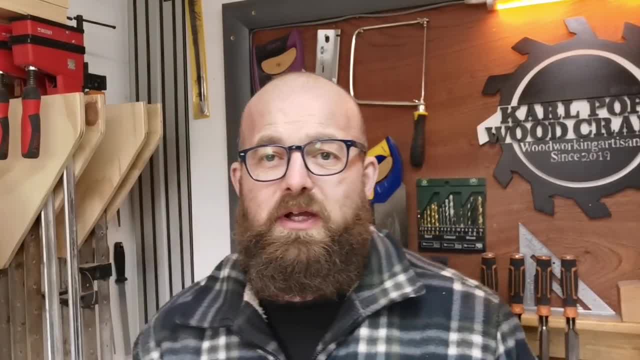 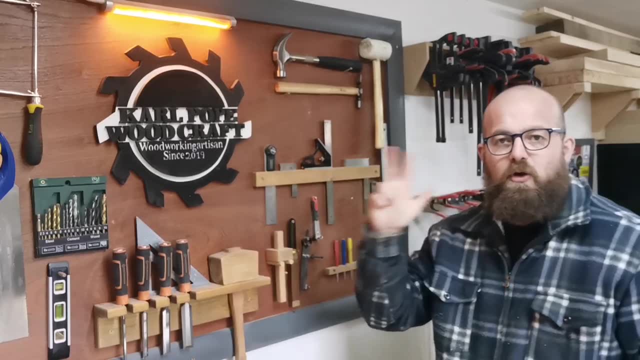 find them all over the place. they're a really good little money area and they keep you going in the times when everything's quiet. so get yourselves on there on xe or ebay, see how much they're going for and selling for a similar sort of price. coming in at number three is the mirrors that i make. 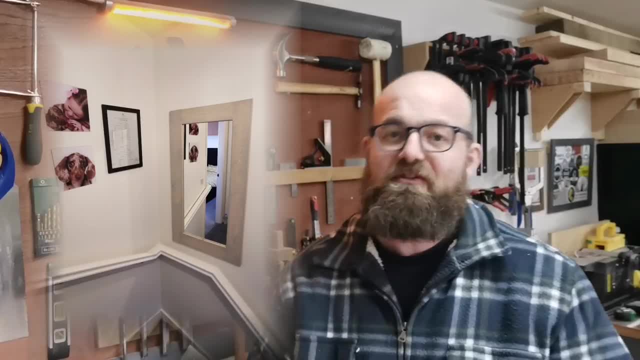 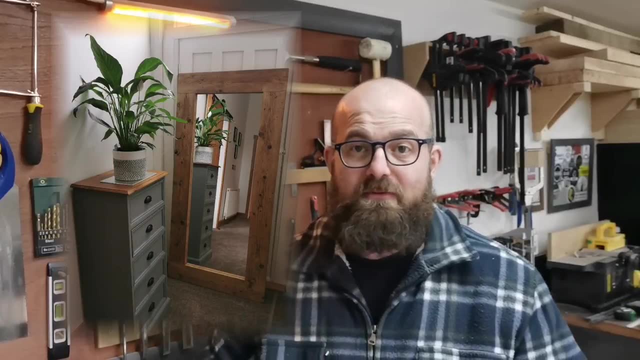 now again, these are pretty simple. to make a little bit more time consuming, you have to little, be a little bit more accurate. but again, i use scaffolding boards or pc plain square edge timber and i just cut them down to the dimensions that the client wants and then i 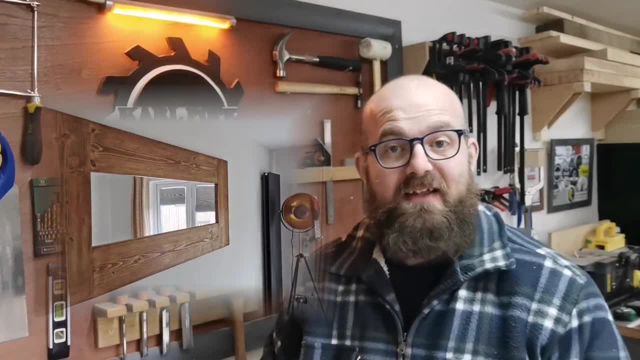 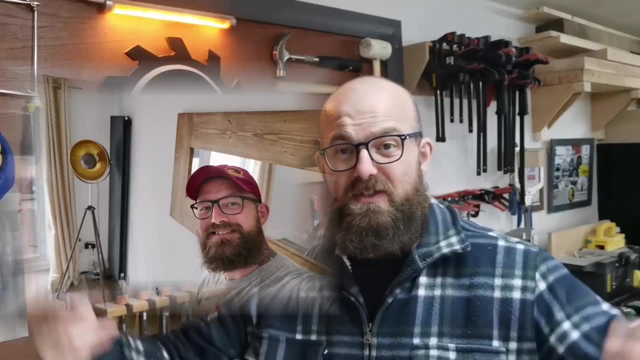 take it to the mirror shop where i buy all my glass and mirrors and things like that from, and they fit the mirror for me. and then it's again so simple: sand down with 80 grit wax. i use pocket holds in the top to attach the boards together and in the bottom put four in each one. so it's. 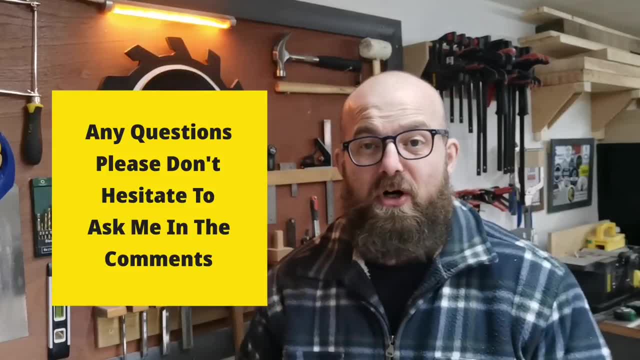 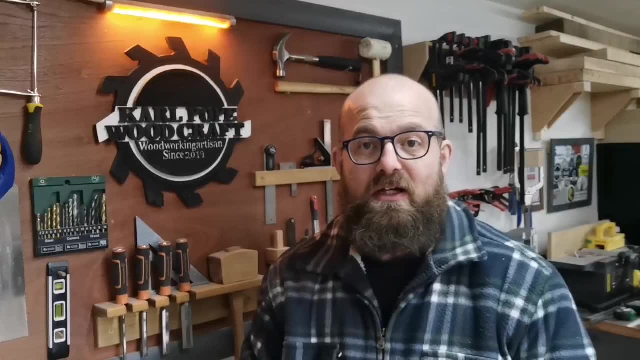 nice and strong with glue and then sand down to 80 grit, put a groove in the back of the board and then take it to the glass shop. they insert the glass into there, pin it in for you, put the safety backing on and away you go and again, these are probably one of the better money earners because 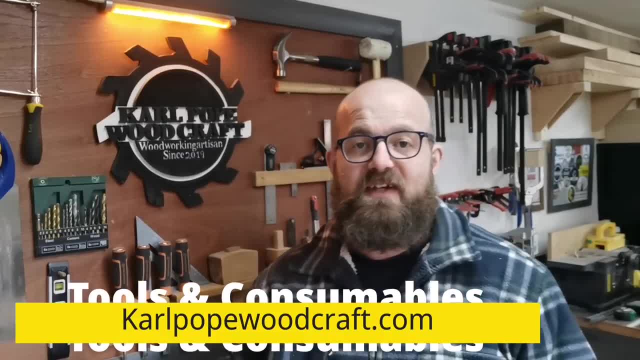 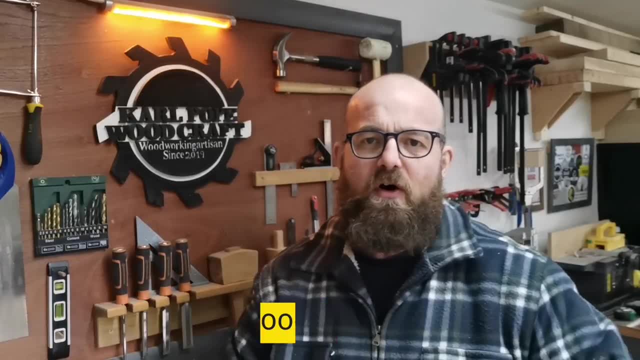 people like the mirrors, want a full-size mirror, they want it bespoke, custom, they want it to fit in a certain place. some of the jobs that you do don't earn as much money as others, and these are the ones that will bump them jobs up. so you can afford to not charge as much for another one, because you win quite a. 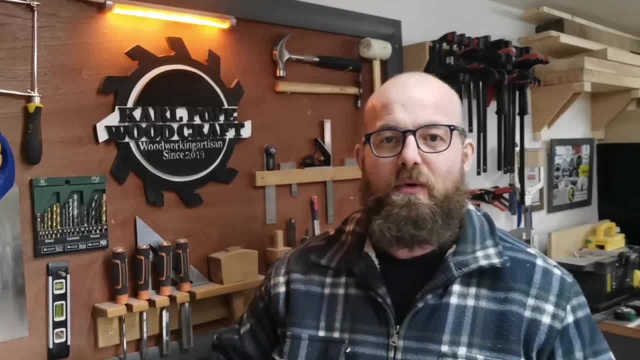 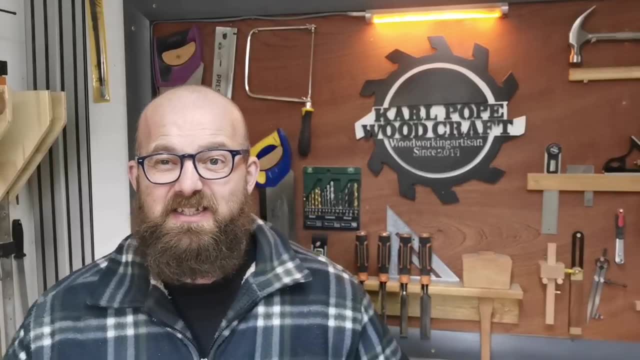 bit off them ones. so all swings in roundabouts and some you earn more on, some you earn less on. and coming in at number two is a really nice, simple one which i like. it's the radiator shelves and this is just. it's just a really good alternative to the old-fashioned radiator cover. 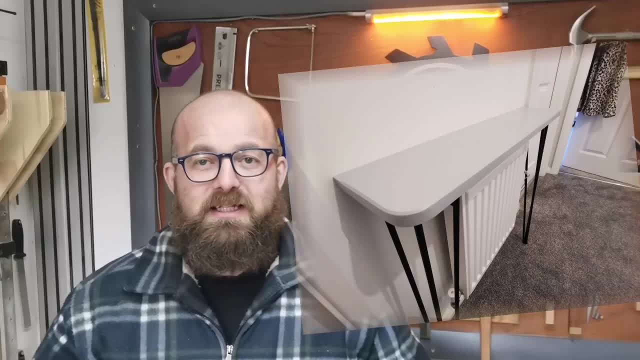 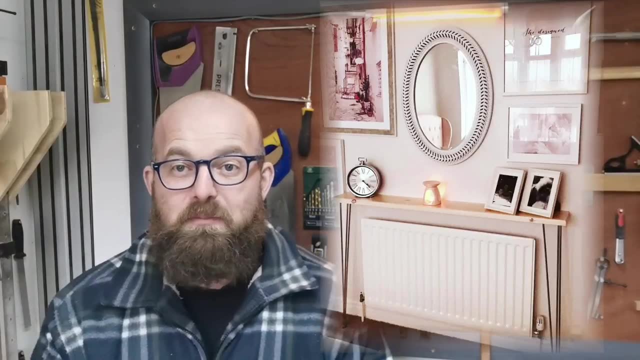 you've got a nice simple shelf with some hairpins legs- really simple. get your client send you the dimensions of the radiator. add 150 mil on either side- i always do mine- 150 deep as well and that should fit any size radiator. i offer a fitting. 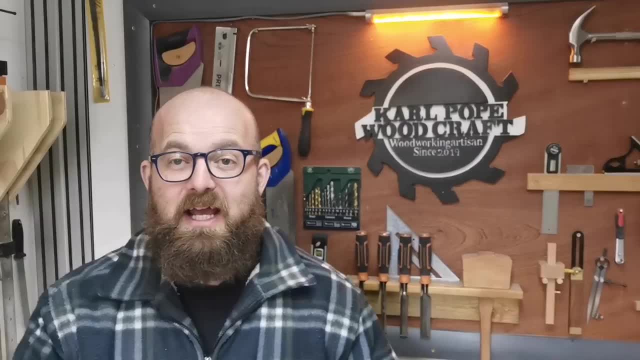 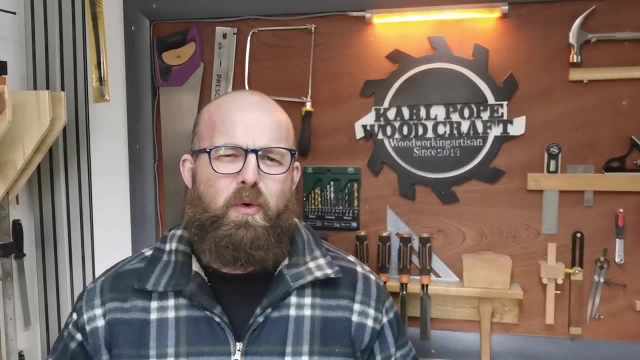 service as well. so i deliver it anywhere in the region where i live and i install it. so it just takes all the hassle out of it for the client. yes, it's simple and you know you can make one of these at home yourself. but what does everybody hate doing? they hate fastening them to the wall. 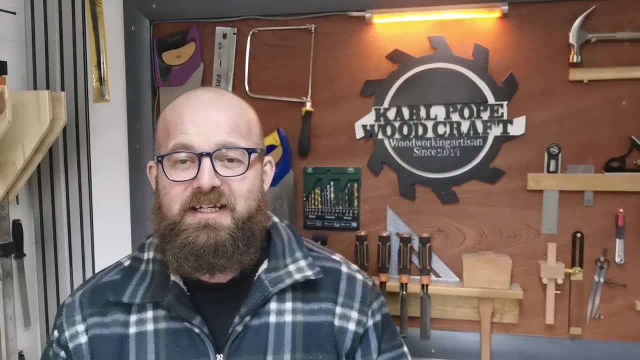 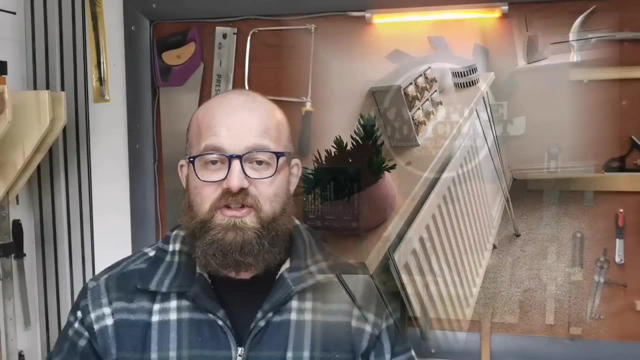 themselves. they hate putting pictures up. they can never get the plugs to work, you know they always have problems getting them aligned and level and stuff like that. so take that out their hands, go around there, install it, fit it free, clean up and then you've got a nice, simple. 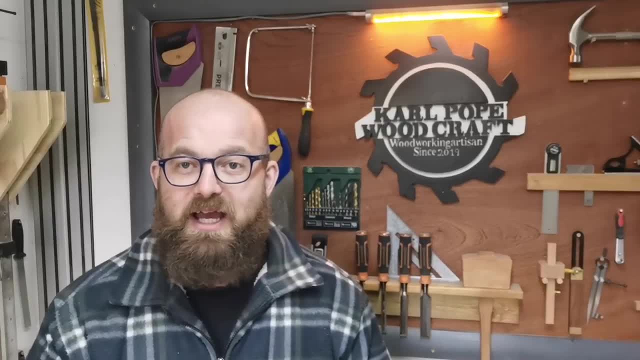 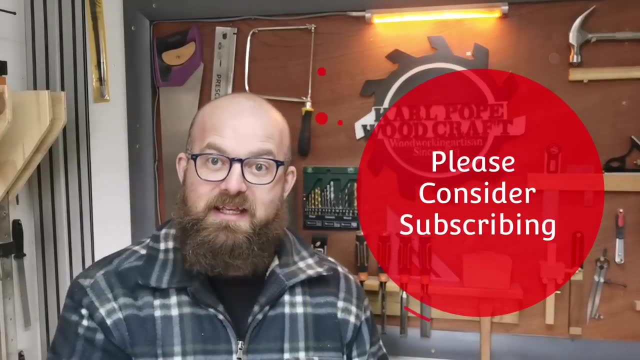 radiator shelf and some hairpin legs- stylish, modern and a good little money earner for you, and it gets your clients looking at the rest of your stuff, which then purchase other things which we'll come on to later in the more into intermediate projects and coming in at number. 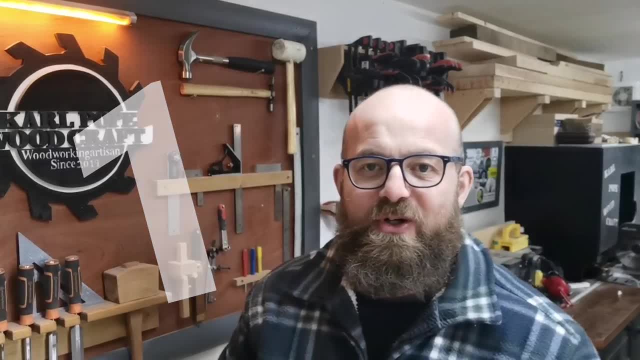 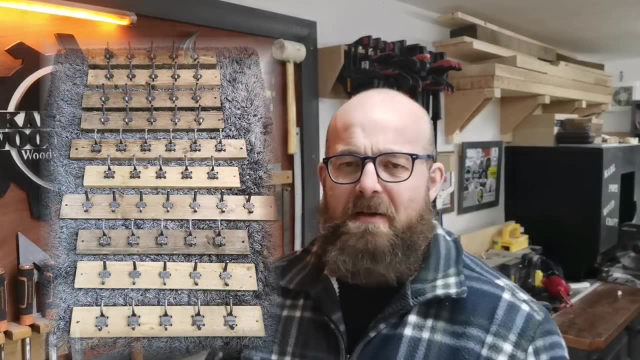 one on the beginner projects is my famous, made in hull coat hooks. now, these are a great little money because they're just so simple to do and everybody wants a solid coat hook because there's no worse than going to one of these diy stores or whatever. yeah, you can pick them up for like 10 or 12 quid. 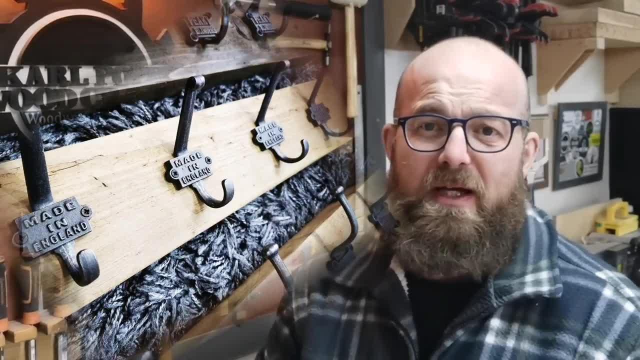 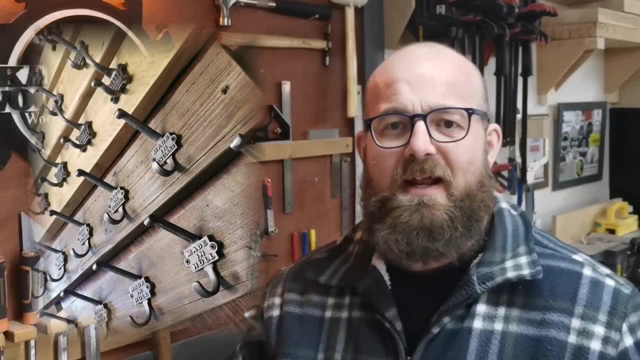 up to 20 quid or whatever, but you hang more than two coats on. snap away the go. so find yourself a good quality metal smith in your area getting to make you some good quality core hooks. put them on a nice piece of solid spruce or pine and put some decent size screws. 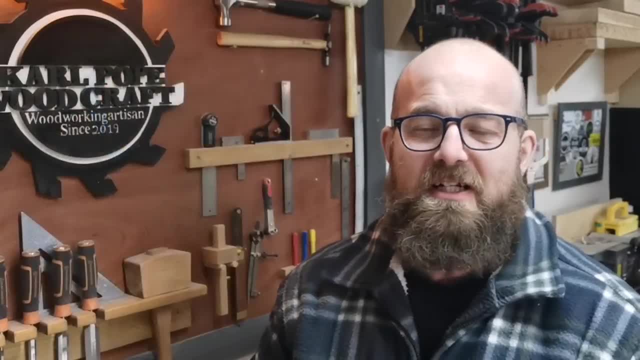 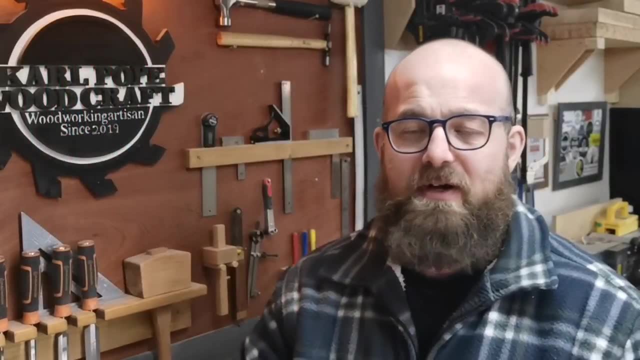 into them brackets, and supply them with some decent screws as well to put it on to the wall. so everything's nice and strong again. really simple to make a piece of pseo, piece of spruce. sand it down to 80 grit, make it look nice and rustic, wax it. we can do anything you can paint.